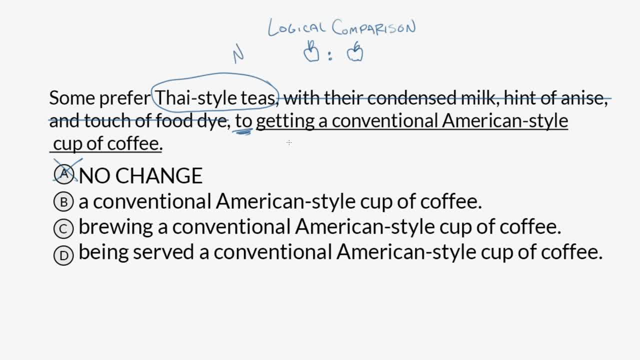 Well, Thai-style teas is just a little noun phrase, Whereas getting a conventional American-style cup of coffee is a gerund phrase. See this ING verb. It's a gerund, It's a verb behaving as a noun, And I can see how this would be a tempting choice, right. 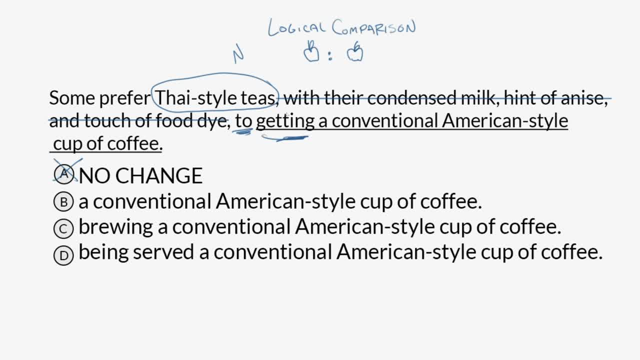 Like a gerund is in its way technically a noun, But what we're doing here is illogically comparing the experience of receiving a coffee right- Getting a conventional American-style cup of coffee- to the idea of Thai-style teas themselves or teas as a category right. 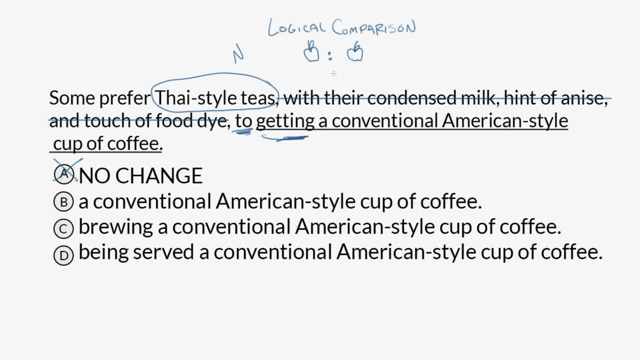 And that's not the same. That's not comparing apples to apples, That's comparing apples to a bowling ball. It's not the same. It's not the same thing. That could also be a coconut, but let's just say it's a bowling ball. 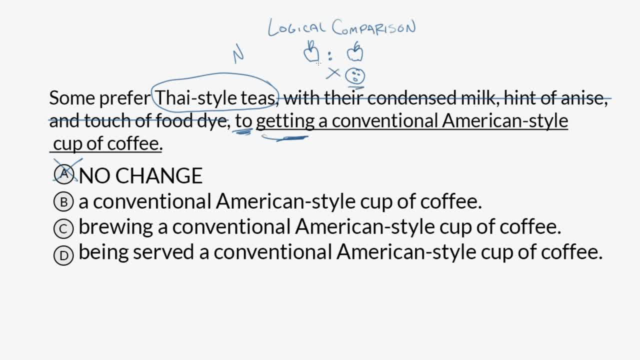 It's not illogical comparison. It's two completely separate classes of thing. So what we're going to want to do as we go through these answer choices is eliminate those options that don't really compare Thai-style teas to an equivalent Option B. some prefer Thai style teas to a conventional American style cup. 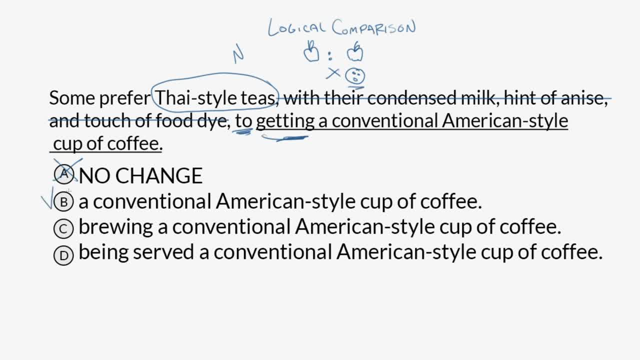 of coffee. This, to me, seems to make sense. I'm going to say this is my front runner right now, because it's not an experience, it's just another noun. It's an American style cup of coffee which contrasts neatly with Thai style teas. But let's confirm that hunch by going on to: 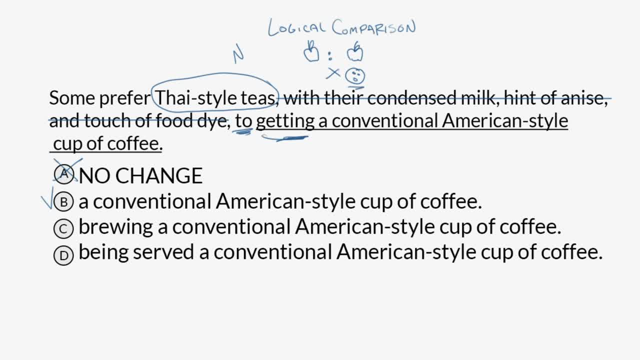 option C and D. So option C: brewing a conventional American style cup of coffee. Well, this repeats the same error as the original choice: getting a conventional American style cup of coffee. right, It's comparing this experience of brewing to the idea of teas, or to teas themselves. 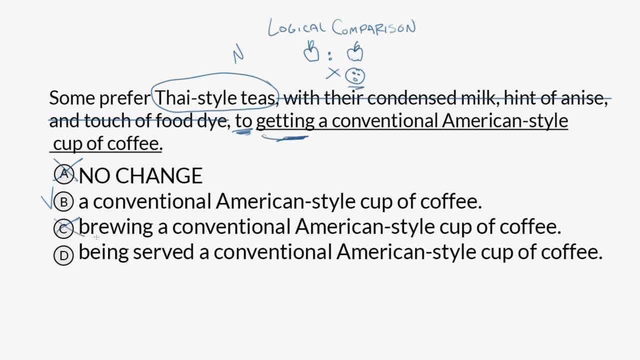 It's not the same. Option D being served a conventional American style cup of coffee. It's awfully similar to answer A getting a conventional American style cup of coffee. And again it's this generalization, This ing word, right, And it's just not. it's not the same. We're not comparing an experience. 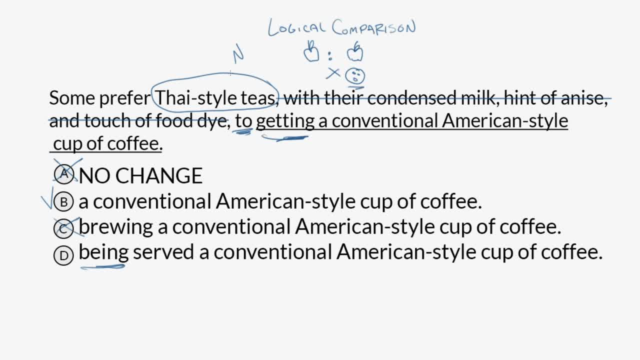 to a tea. We're trying to compare one hot beverage to another hot beverage And ultimately, that's why I want to go with option B, because it correctly compares a beverage to another beverage, And that's what you want to do with a logical comparison question.